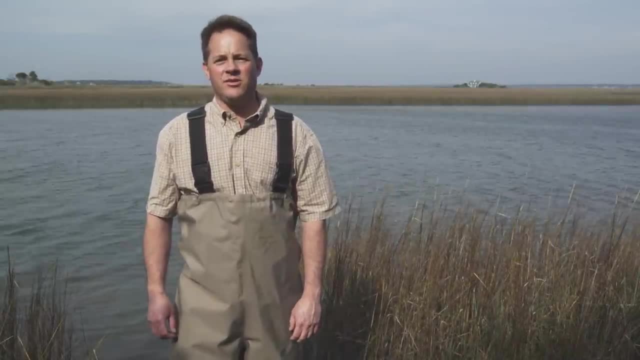 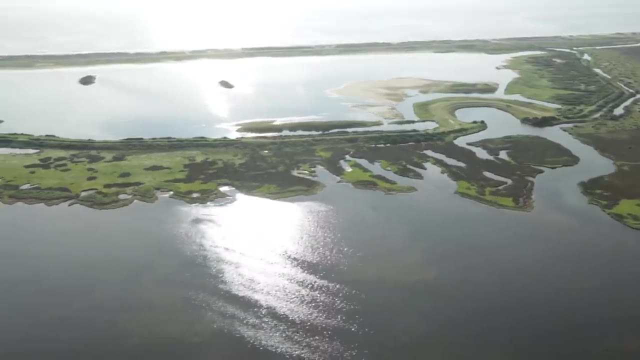 the place where the land and the water intersect on their way to the ocean. Watersheds drain to rivers, Rivers transport materials in the water to the coast and when the rivers meet the coast, they begin to widen out. And in this area where they widen out and begin to interact with salt, 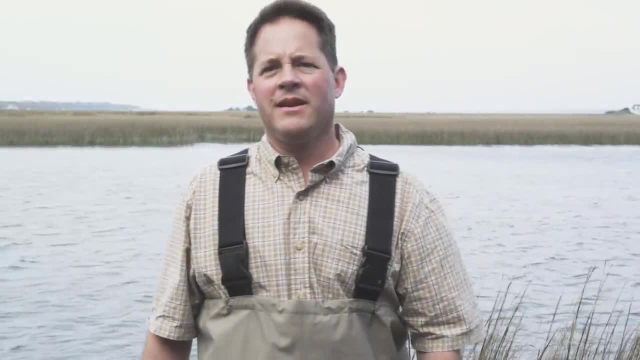 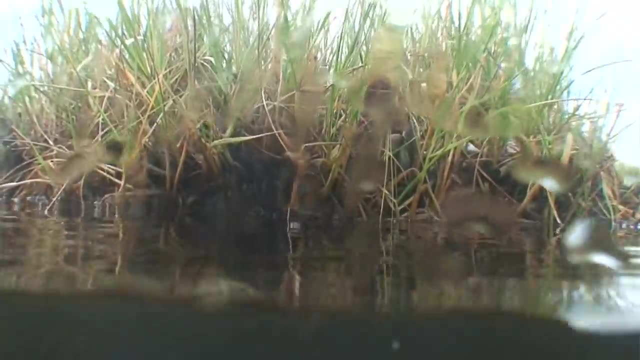 water is an estuary. Estuaries are definitely not homogeneous. People think of them as one thing, but if you look through the estuarine gradient, there are multiple habitat types. The most obvious difference is water depth, but the depth of water determines the way that the 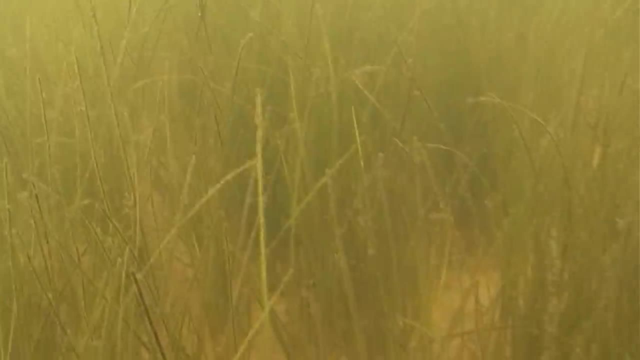 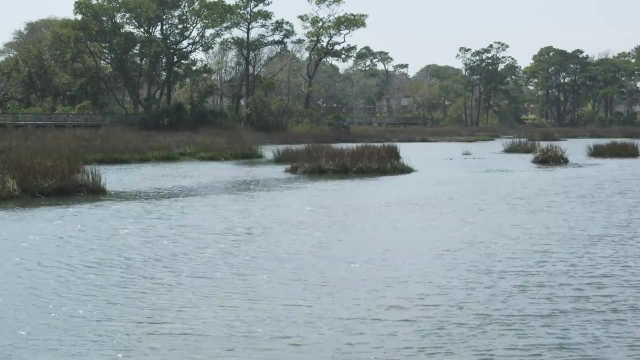 system functions. If you have very shallow water, you can have photosynthesis on the bottom. If you have deeper water, you only have photosynthesis in the water column. Along the fringes of estuaries, such as one where we're standing now, are lots of different habitats. 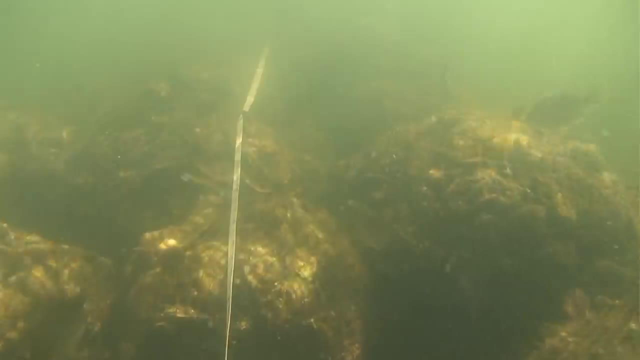 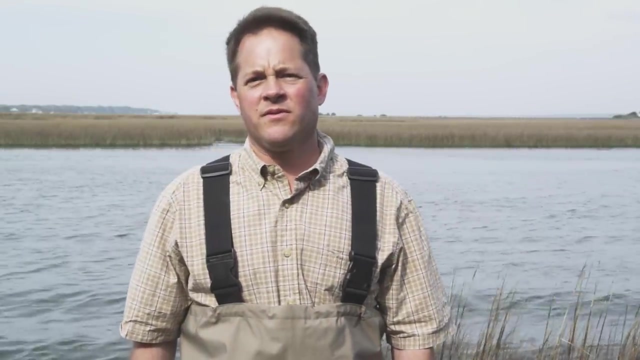 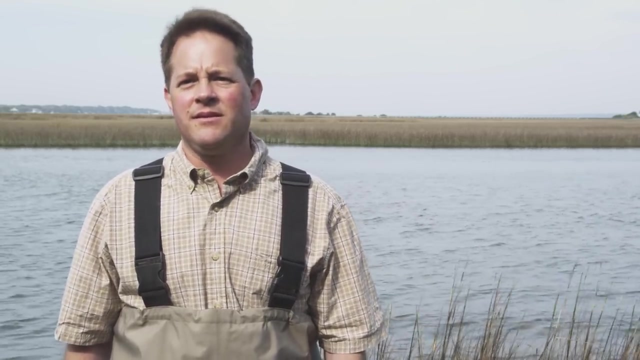 including marshes. As you get farther down into the salty areas, you have seagrasses and you also have oyster reefs. It's important to study estuaries for several reasons. First and foremost, they're a really important area for productivity and processing of materials in aquatic systems. 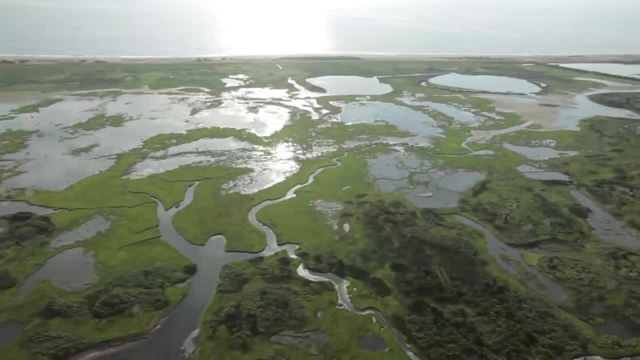 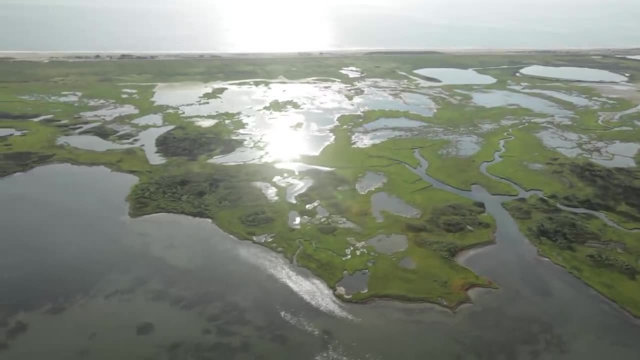 to understand what's going on in an estuary is essential to understand the connection between the land and the water. So if we don't study these processes and see how they're working, we won't know the things that they are doing. that may be of value to us and 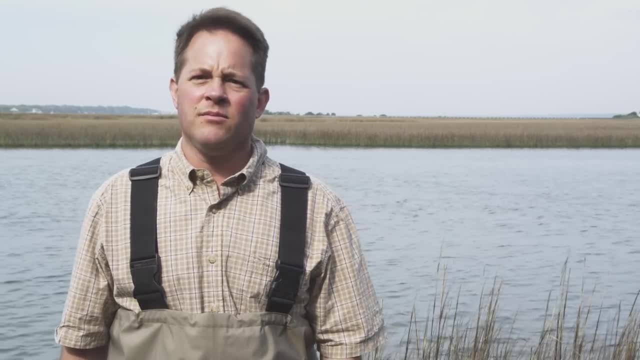 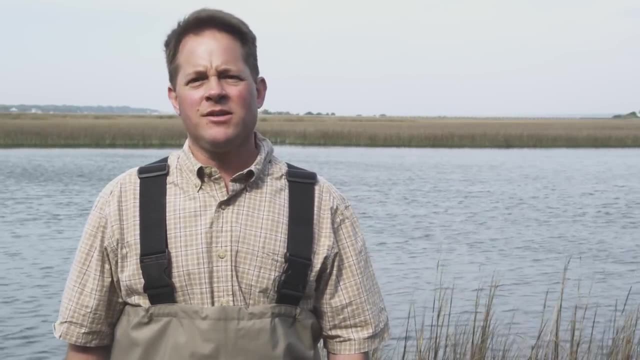 we also won't know the processes that were occurring that may be lost as humans continue to affect the landscape. We've been doing a whole lot of work on oysters. They are important in ecosystem function in that they clean the water column and they transport materials. from the water to the sediments. They also change the way that nutrient cycling occurs in sediments. There has been a lot of faith put in oysters to help enhance water quality, and oyster restoration is being employed as a tool in many systems in which they are trying. 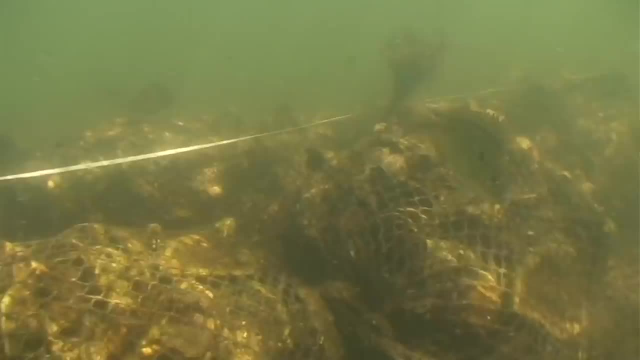 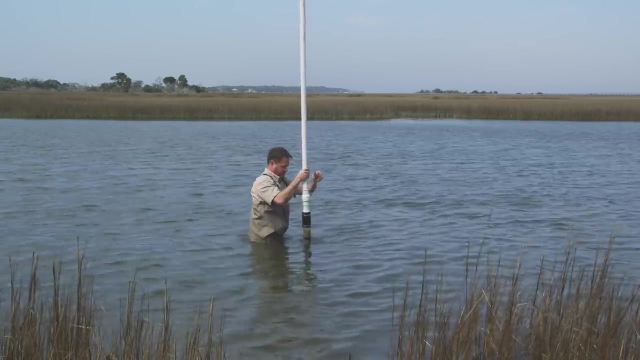 to enhance water quality and combat the effects of eutrophication. We're really interested in the specific processes that oysters stimulate in the sediments. Rather than just think that the what, the material that goes from the water column to the sediments, it's important to think: 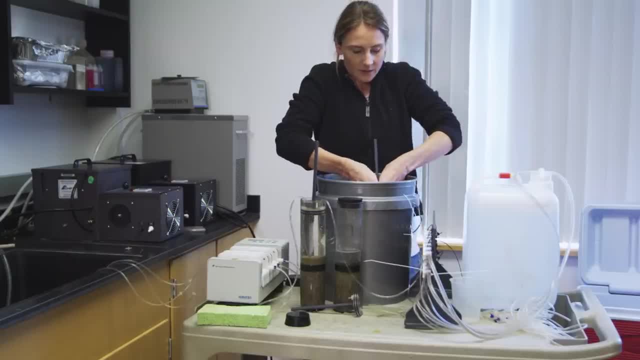 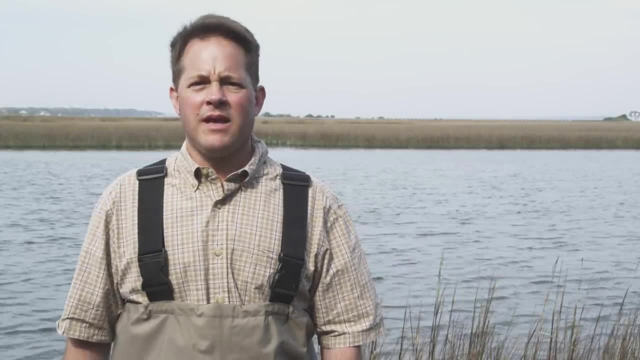 about following proper gradient tourist assessments As the sediment's loss. we like to know the exact fate of that material. That involved some pretty involved experiments assessing specific processes such as denitrification Oysters. as they couple the water column and the sediments, enhance organic matter, They